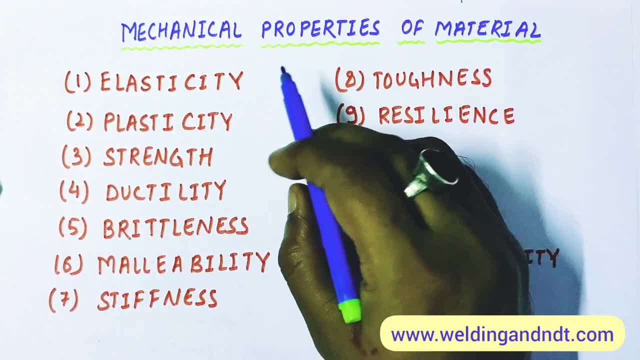 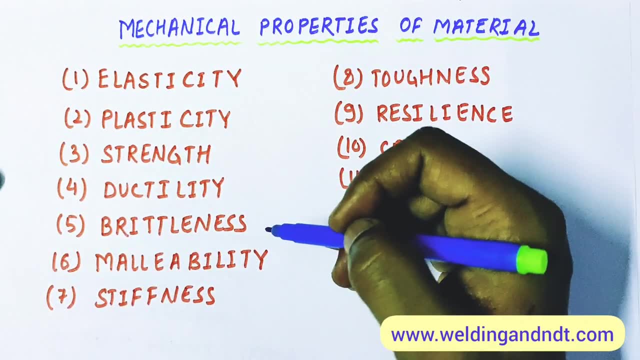 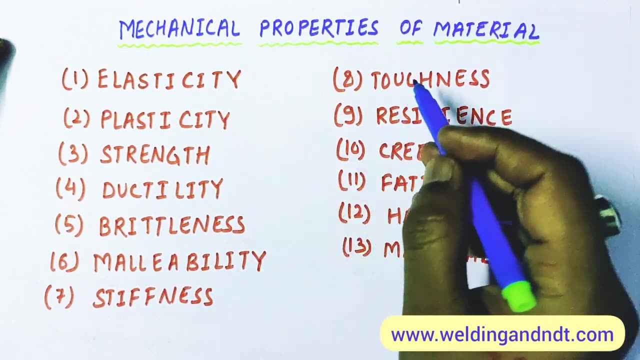 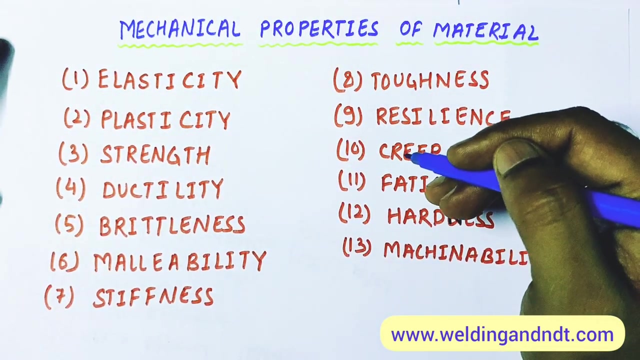 hello friends, welcome to my channel: welding and entity. our today's topic is mechanical properties of material and we'll learn 13 different, very important mechanical properties of material, that is, elasticity, plasticity, strength, ductility, brittleness, malleability, stiffness, toughness, resilience, creep fatigue, hardness and machine ability. so these are the 13 properties which 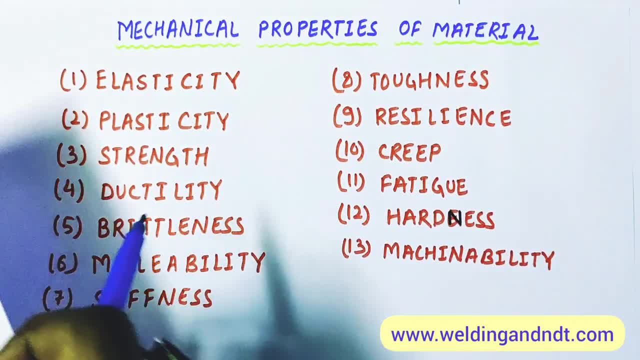 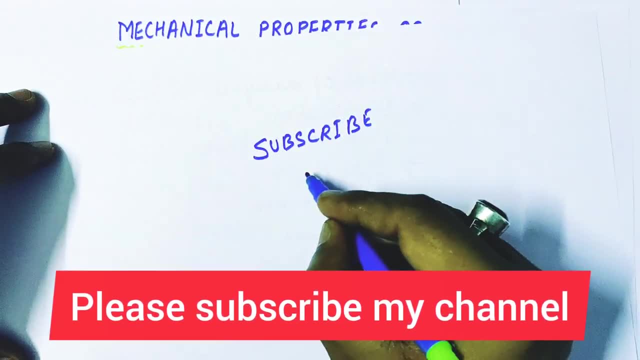 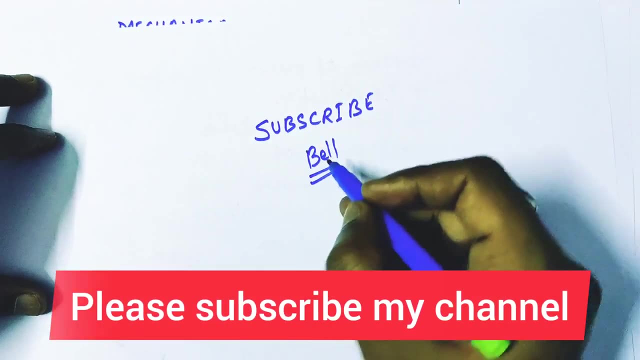 we will discuss today. but before starting this topic or video, i would request you to please subscribe my channel if you have not done it yet, and also please press the bell icon on the right side of the subscribe button. so what will happen if you press the break? 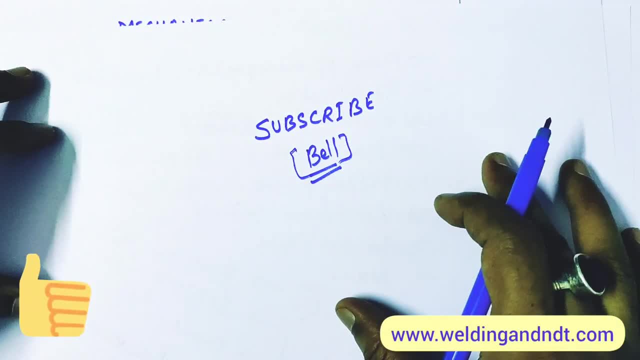 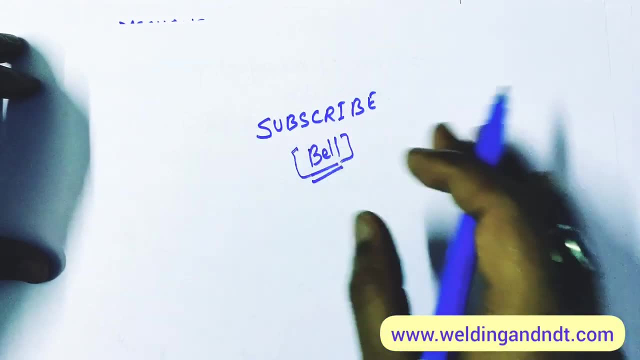 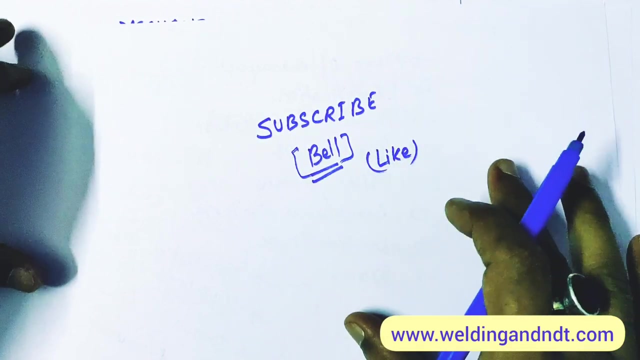 bell icon. you will get regular updates on my new videos, and i used to post videos every two, two videos every week, so you will get regular updates of my videos and friends. i would also like to request you to, please, you know, like this video and share the link with your friends also. so if you find this, 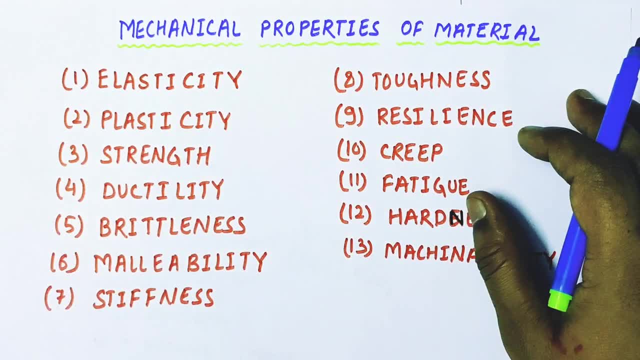 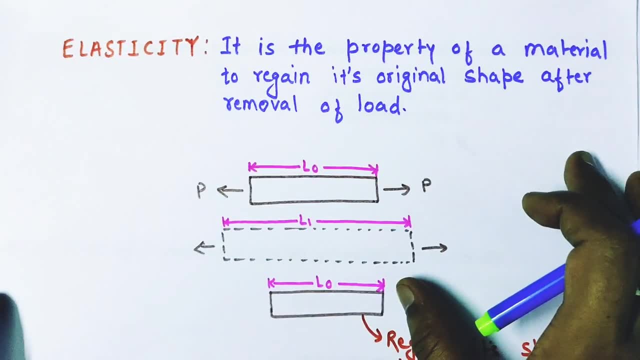 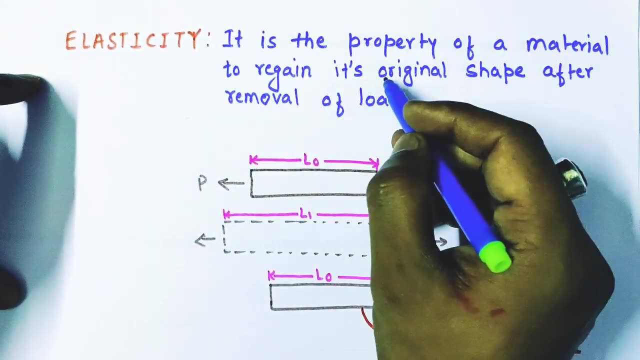 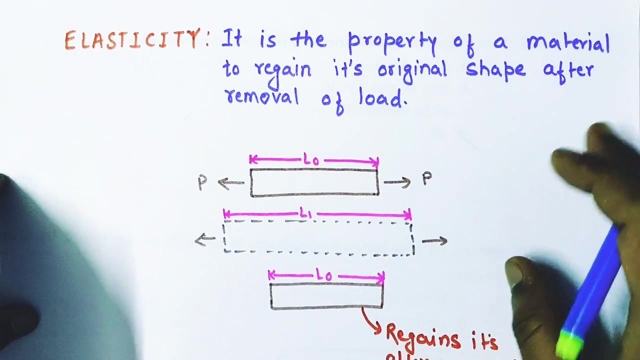 video useful, please hit the like button and share it with your friends. so, friends, we will start with the first uh topic, that is, elasticity. now, elasticity, see elasticity. it is the property of a material to regain its original shape after removal of load. what happens, friends, if we apply some external load, on a, for example? here we have a material and we are applying 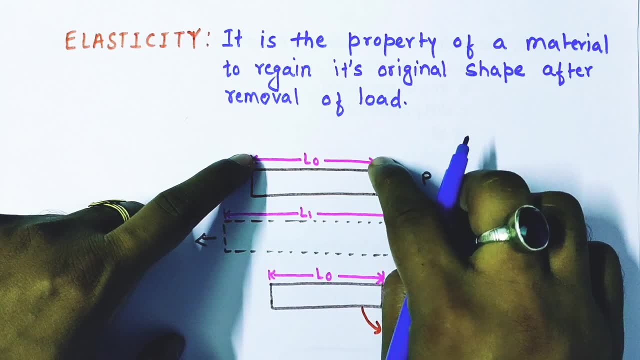 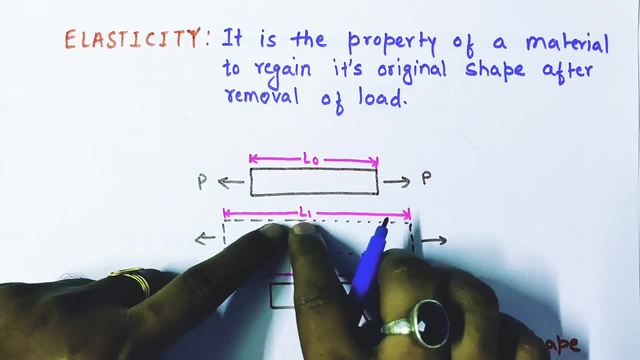 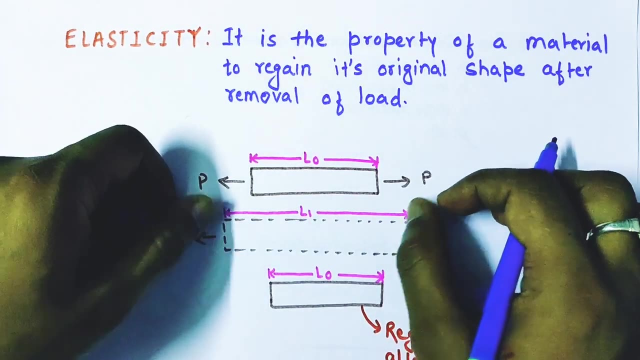 a external load, that is p, on this material. the initial length of this material is a lot now just for, uh, you know. take, for example, if the length of this material increases to l0 due to that external applied load, the length has been increased means the material has been deformed. but if we remove, 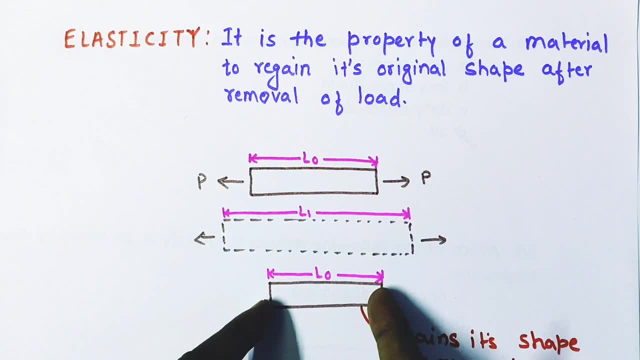 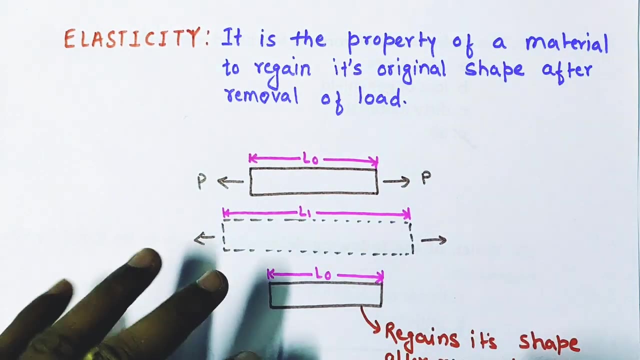 and if that item comes back to its original shape, then we'll say that that material is elastic or the material is showing the elasticity property. means, after removal of the load, material has regained its original shape. here I have written also regains its shape after removal of load. means the original. 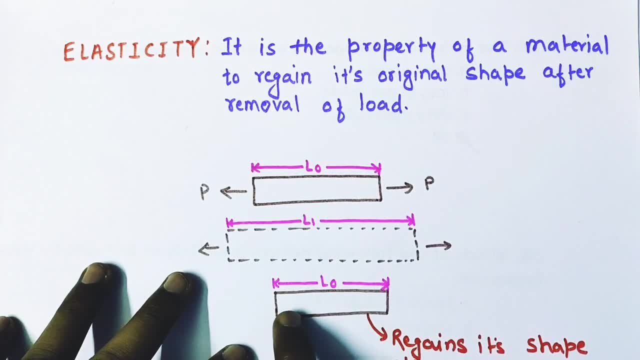 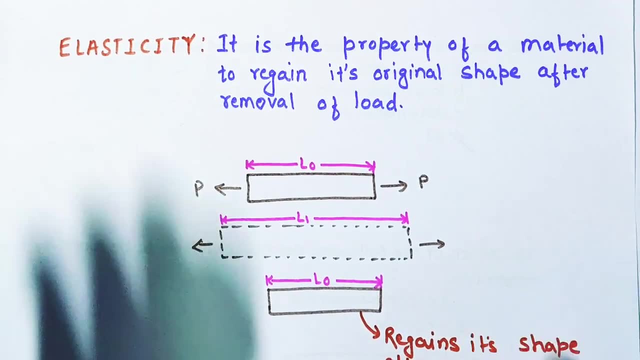 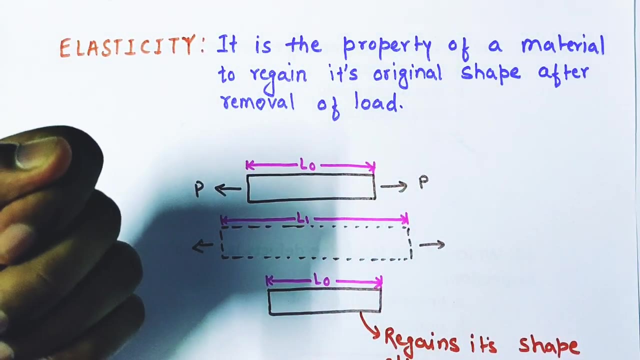 length was a lot, and the final length after removal of the load, is also a lot. hence, material has regained its original shape. we can understand the property of elasticity by a rubber band. so imagine if you, you know, pull the rubber band apart. what will happen? the rubber band will deform, but as soon as 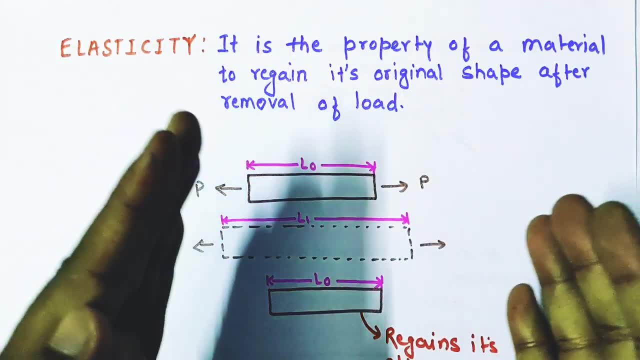 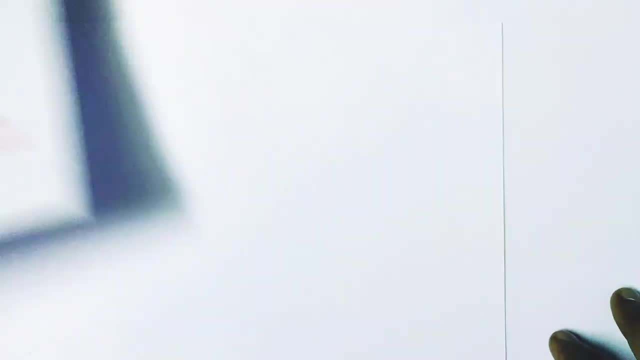 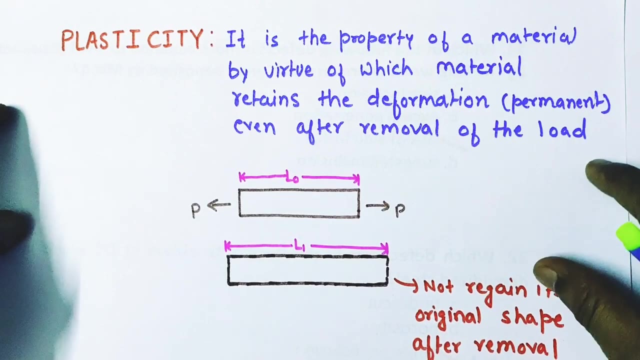 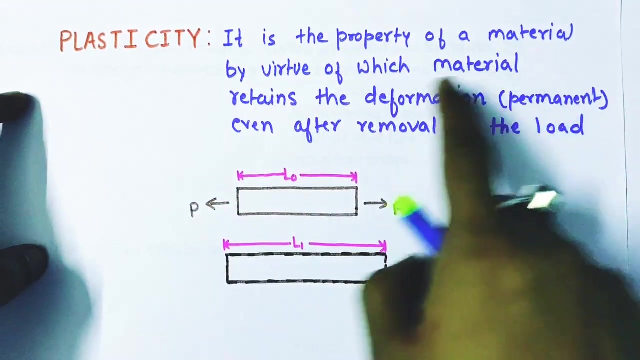 you remove the load from the rubber band, that rubber band will come to its or it will regain its original shape. so that is elasticity. now, after elasticity, will understand elasticity. so what is plasticity? plasticity, it is the property of a material, by virtue of which material retains the deformation permanent, even. 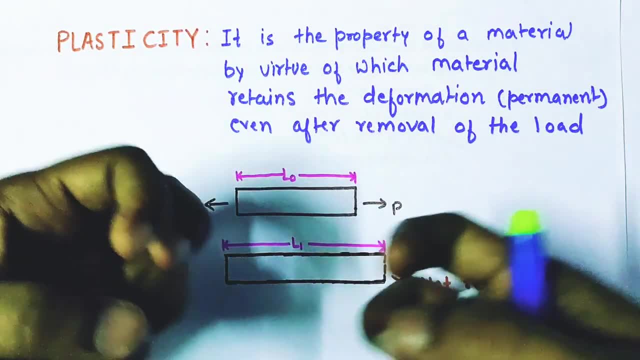 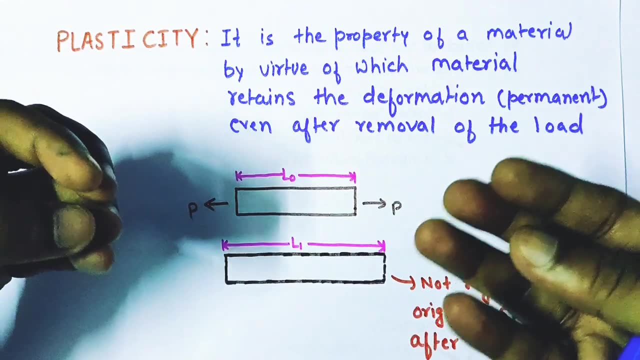 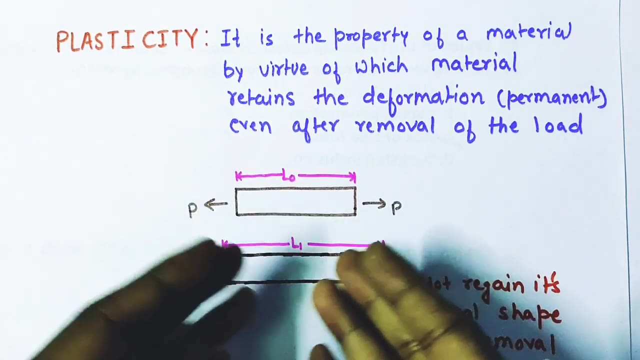 after removal of load. so what happens if we pull a material apart by a load? so it will deform. but if, when you, you know, release that load on or when will you remove that load? if the material will fully release, it will release the load load. if the materials doesn't regain or doesn't come back to its original shape, then we will show. 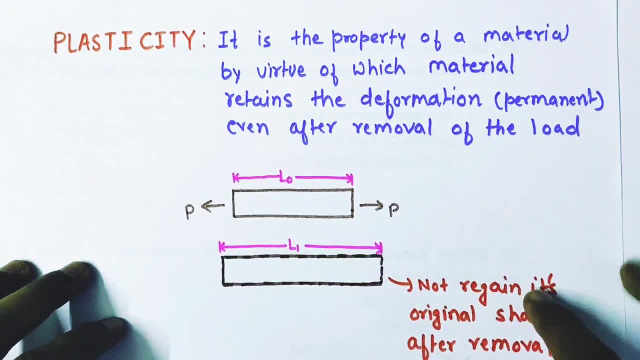 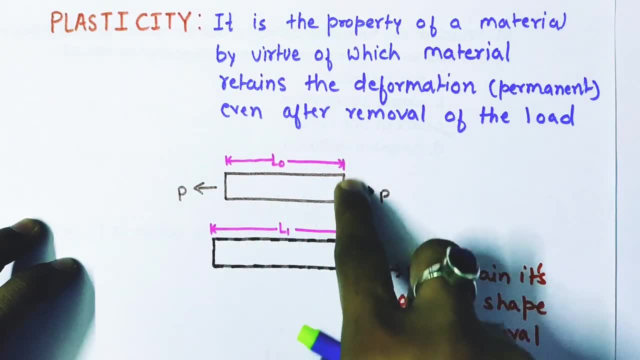 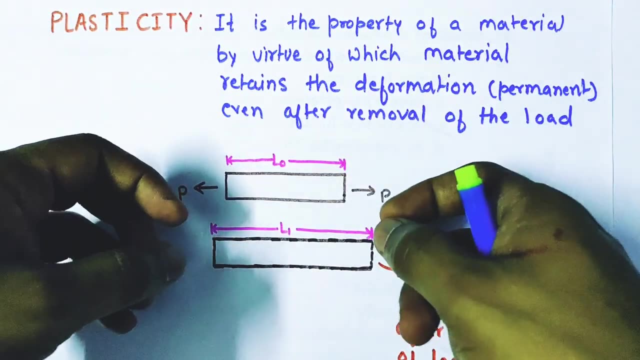 that the material is showing the property of plasticity means not regain its original shape after removal of load. see here, for example: i have taken a material and i have applied a load p, so the original length of this material is l, not now after application, after pulling that material. 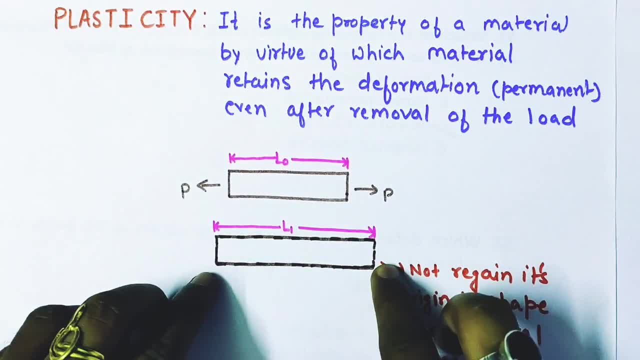 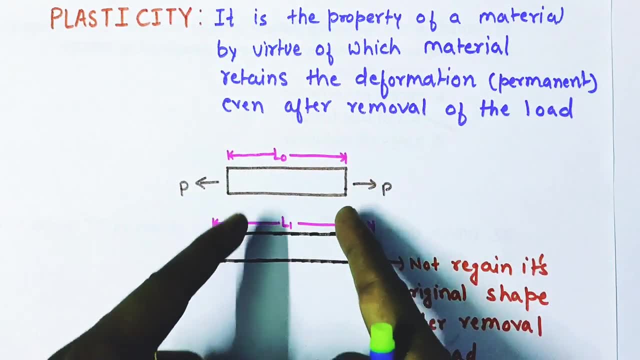 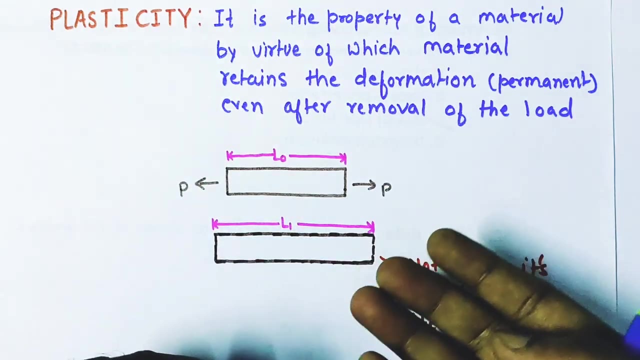 by load p, i have removed that load. but even after removal of the load, the material has not regain its original length or has not regain its original shape. hence i will say that material has undergone a permanent deformation. so permanent deformation after removal of load is nothing but. 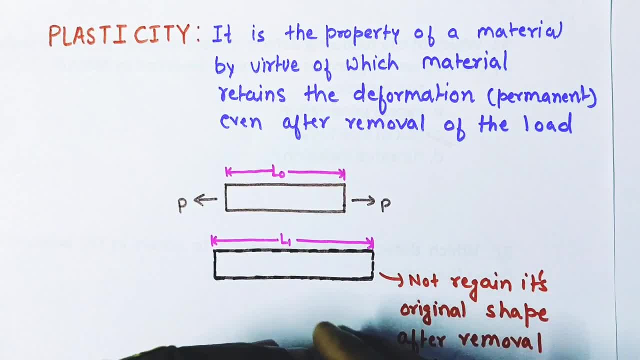 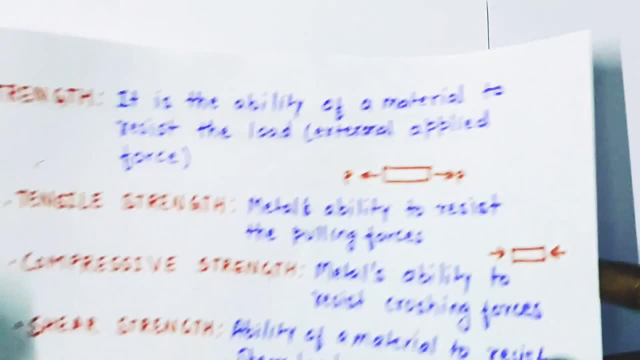 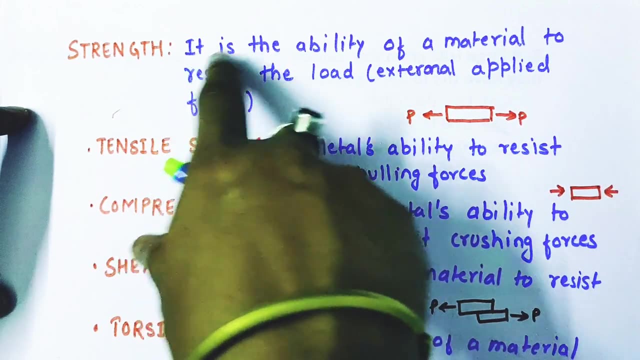 the plasticity. hence i'll say that the material is showing the property of plasticity. so this is plasticity. now we'll move forward. the third important parameter, third important property: strength. so strength is nothing, but it is the ability of a material to resist the load, that external load. 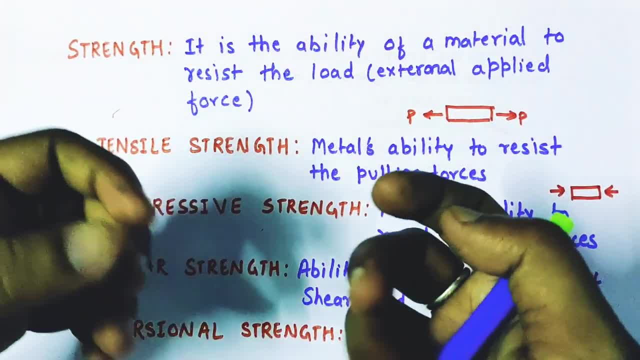 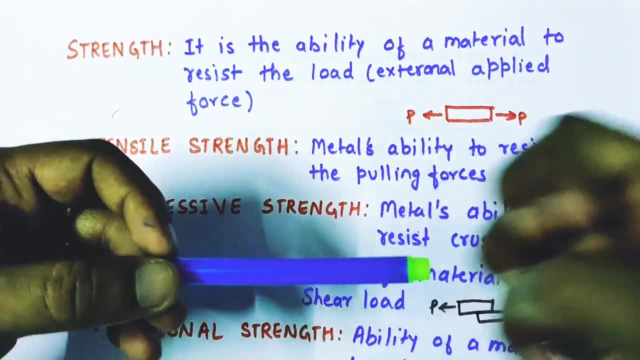 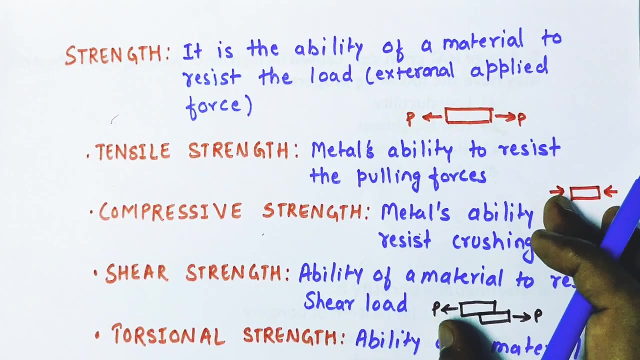 suppose if we apply some external load on a material, this is a material, and if we apply some external load, so this material will resist that external load to a bit, so that resistance of the external load is known as the strength. now there are four types of strength: tensile strength, compressive strength, shear strength and 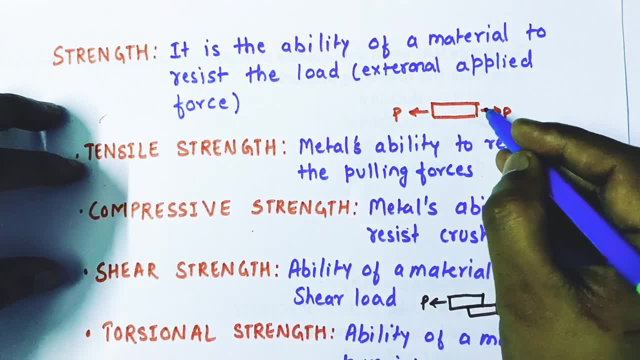 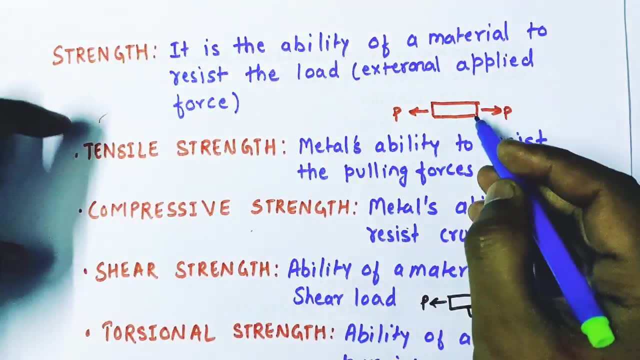 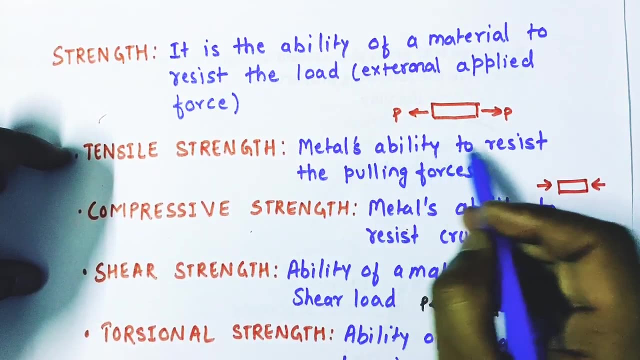 torsion strength, tensile strength, if suppose this is our material and if we pull that material, pulling this material apart. so this is, this type of force is tensile force or tensile strengths, and the strength will be tensile strength. material ability is to resist the pulling forces. 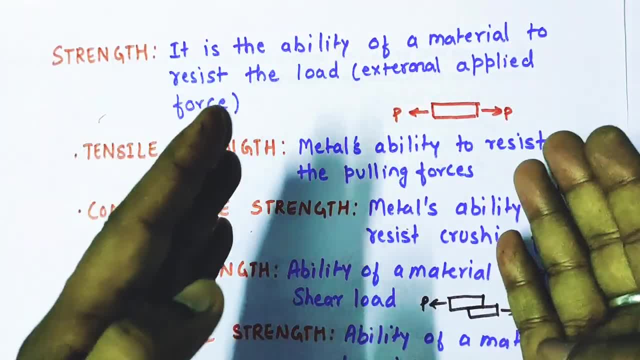 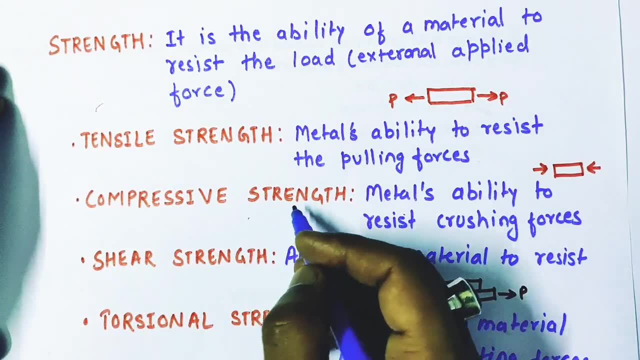 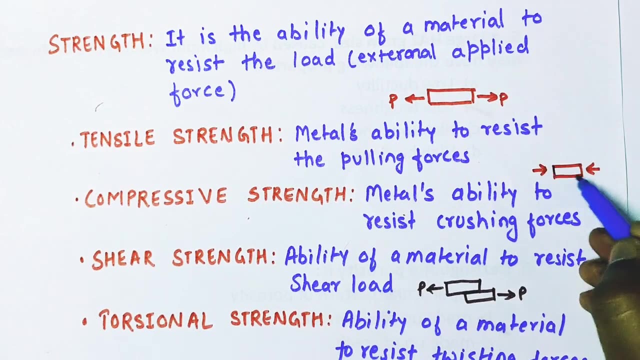 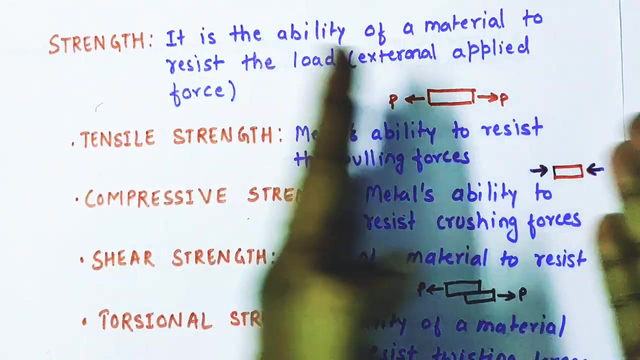 if we are peeling, pulling the material, and the resistance which the material will offer against the pulling will be known as tensile strength, then compressive strength. so compressive strength is nothing but crushing metals. ability to resist crushing force like this is our material and we, if we apply load in this manner, not apart, but in crushing sense. so 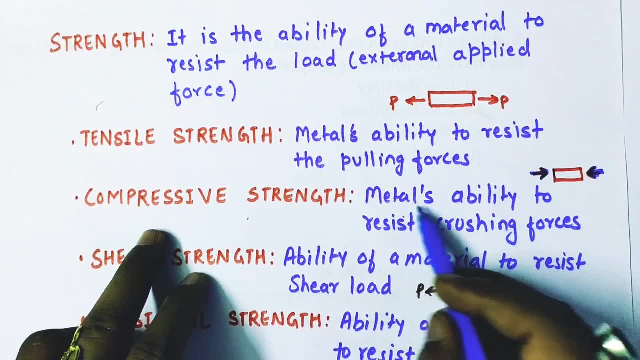 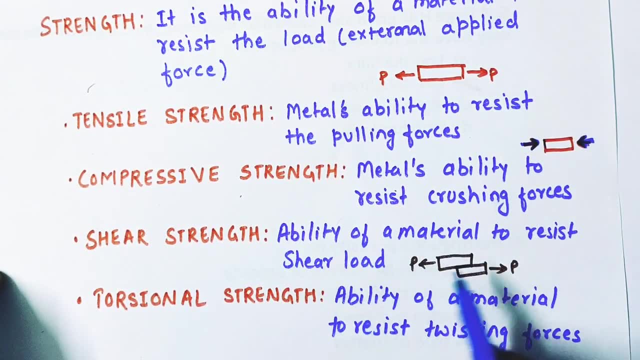 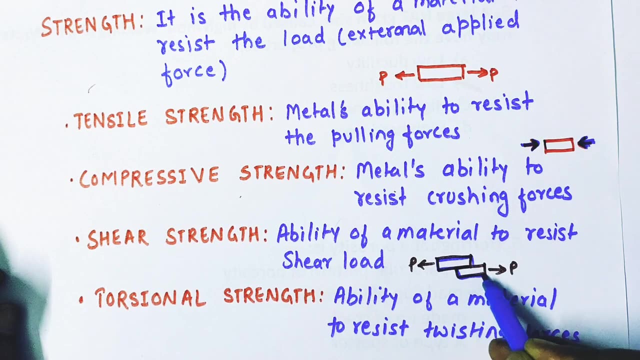 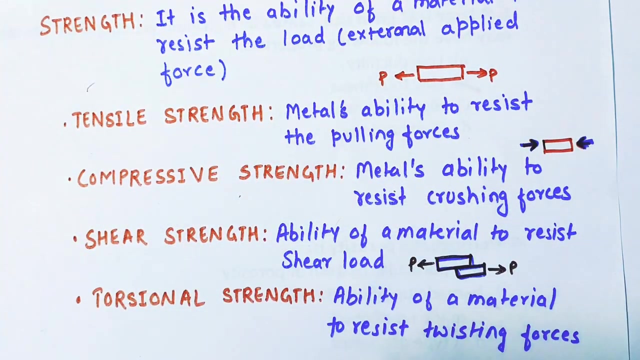 this is crushing force. so materials ability to resist this crushing forces is known as compressive strength. now shear strength, ability of a material to resist shear stress. shear stress is nothing, see, if we have a two material, like one material here and the other material in this manner. so the sliding force, see the sliding of the material- is also, it also creates. 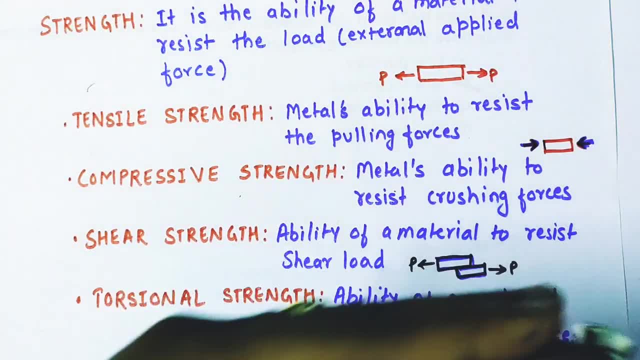 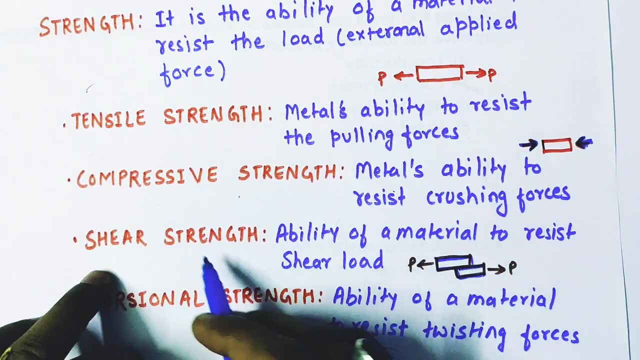 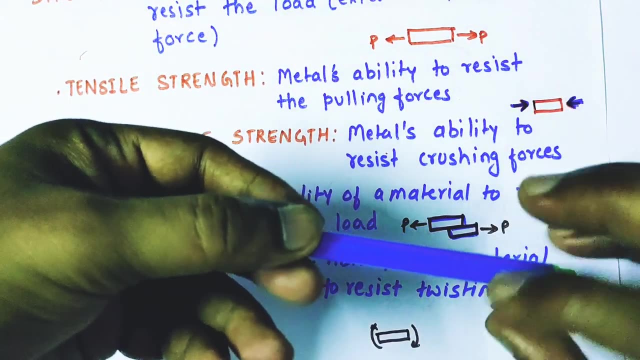 you know, force, so that this force is shear force. so the ability of material to resist the shear load, this type of loading is shear loading and the strength will be called as shear strength, now torsion strength. if there is twisting force, like the in this sketch pen, there is, will be one twisting force in this manner and other twisting. 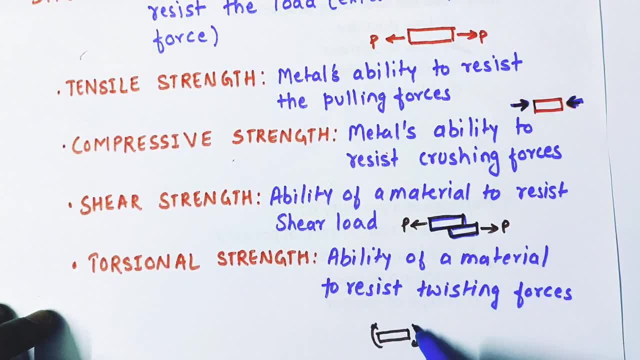 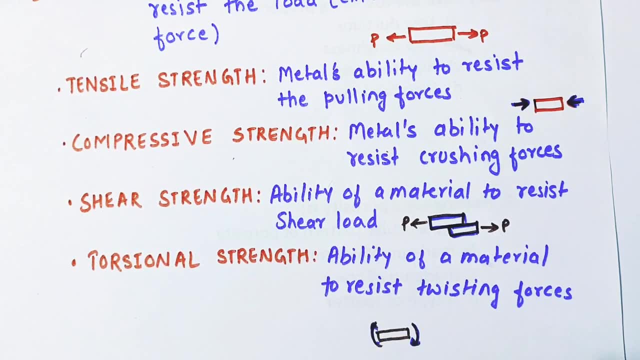 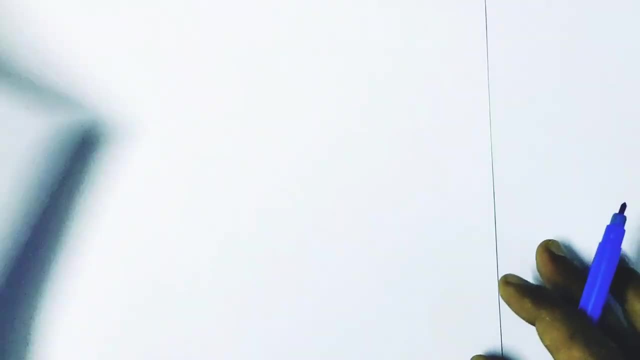 force in this manner. so the ability of a material to resist twisting force- see here in the diagram also twisting force- so more the material ability to resist the twisting force will say that material degree. so this long twisted force means the tension of material in this manner and other twisting force. 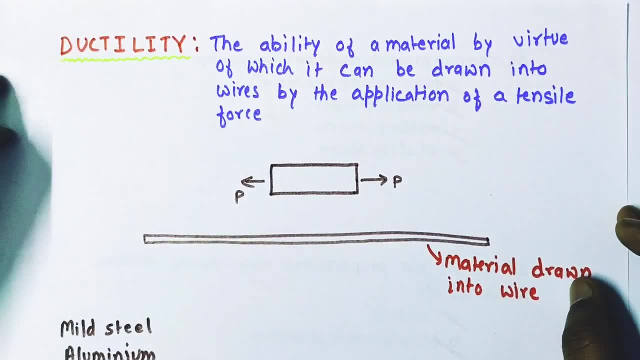 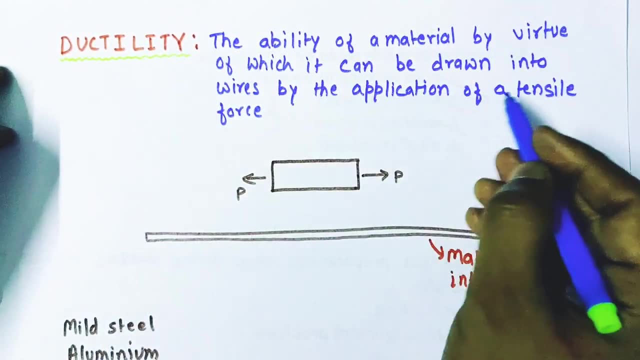 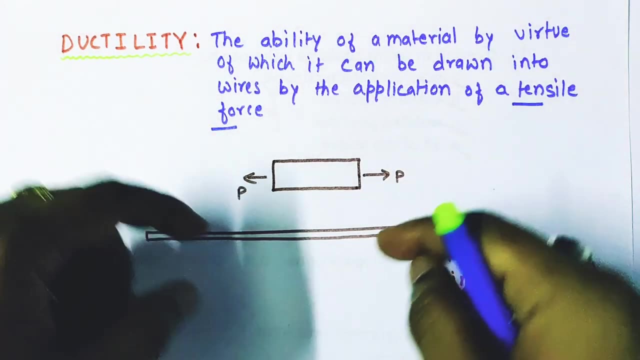 so material utility is also a gravity relationship, but still, material utility is also a constant. the material'' now, after strength, will move to ductility, The right form. it is one of a very important property of a material. Ductility is the ability of a material by virtue of which it can be drawn in to wires by the application of tensile force. 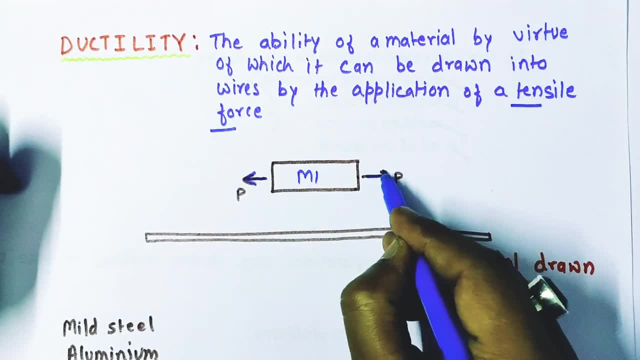 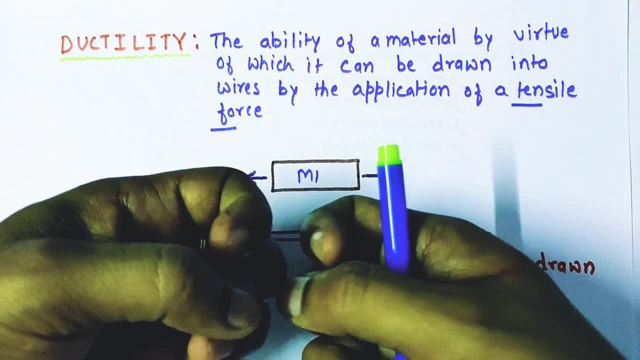 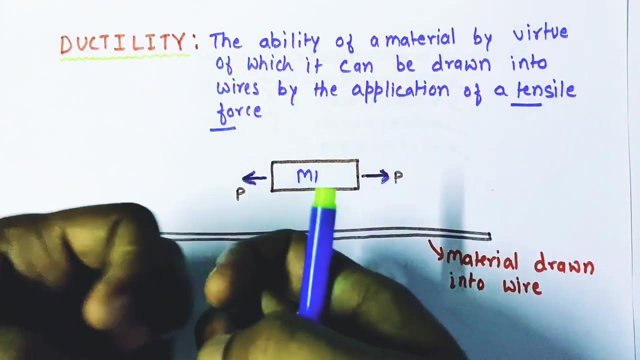 Here you remember this tensile force. The tensile force is nothing but pulling the materials apart. forces are pulling this material. now what will happen? if the material will be ductile, then if you pull this material, that material can be drawn into thin wire and it will come, go on, you know, go on forming or go on becoming a thin wire. 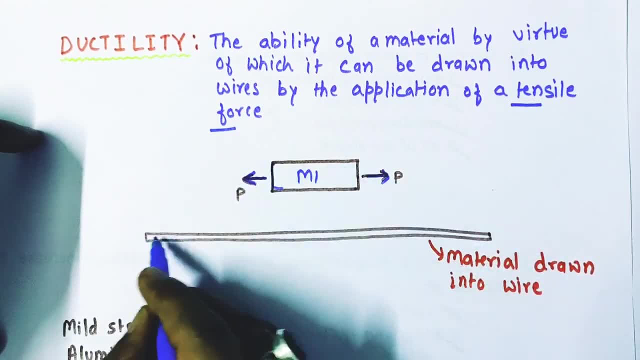 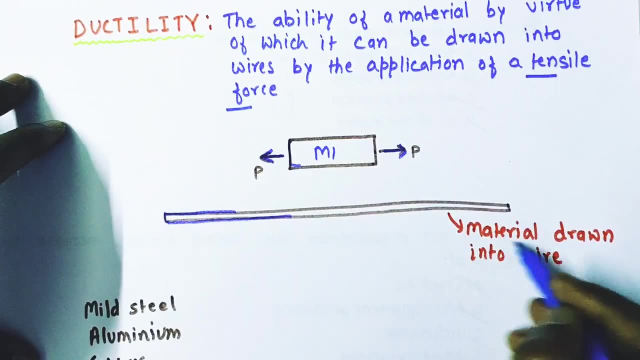 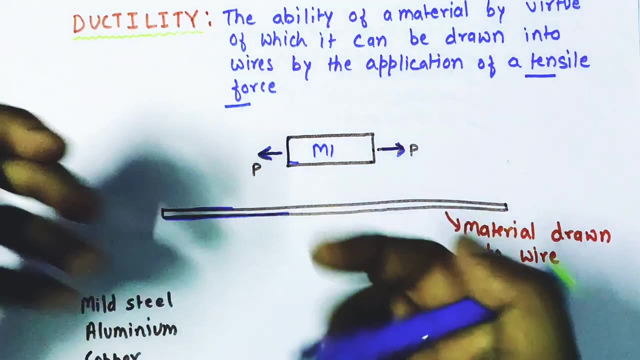 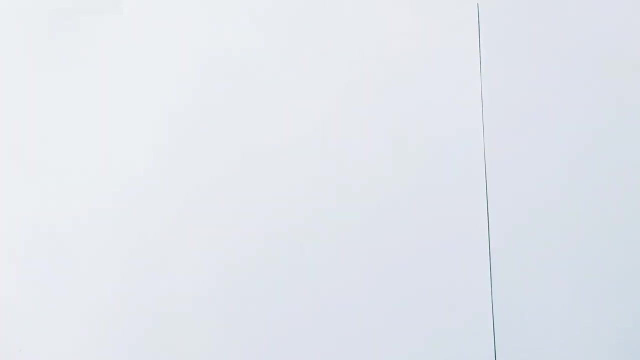 like this. initially the size of the material was this and after pulling this material it has formed into a thin wire. here: material drawn into thin wire. so the more the material can be drawn into thin wire, we will say that material is more ductile. mild steel, aluminium and copper are some ductile materials. now, 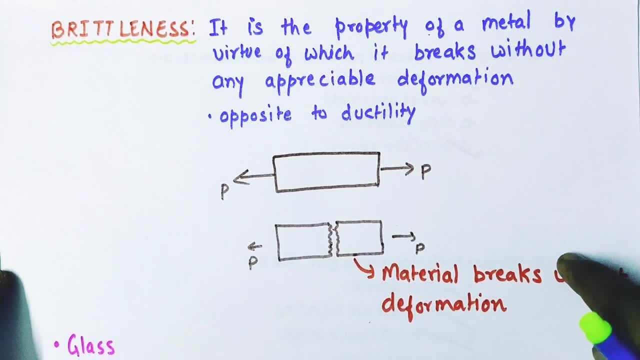 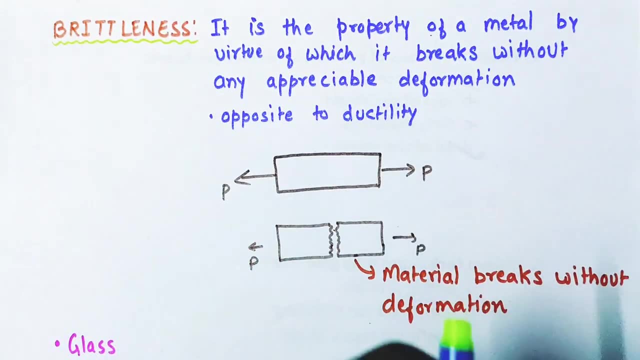 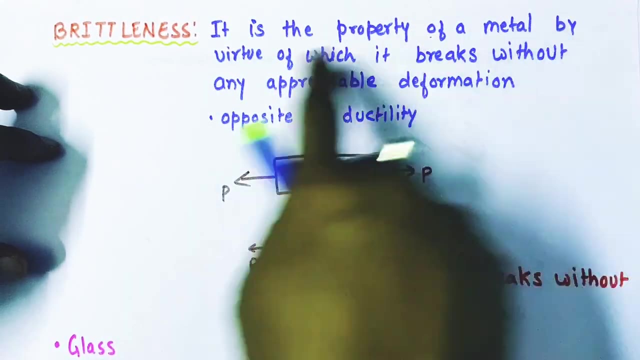 we'll study brittleness. brittleness is opposite to ductility, see. in ductility, the material can be converted into thin sheets while applying external load. but in brittle load- see first let us read the definition- it is the property of a mud tail metal, by virtue of which it breaks without any appreciable deformation, without any 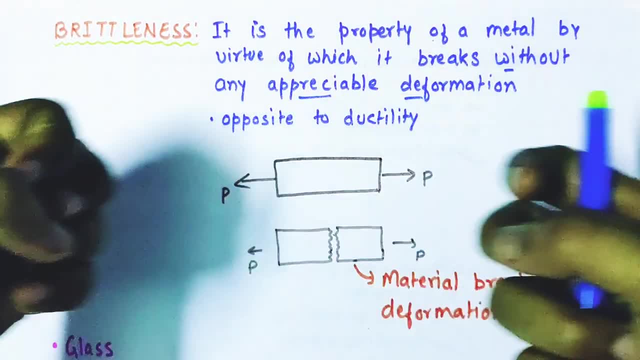 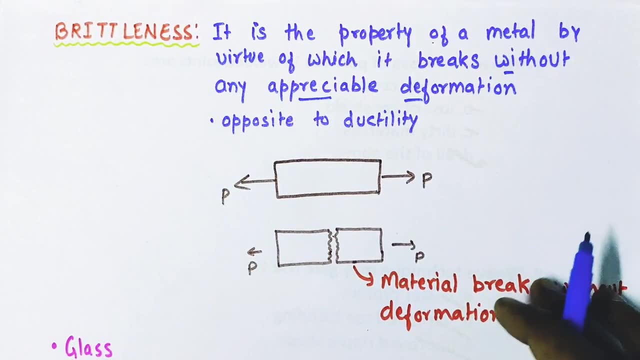 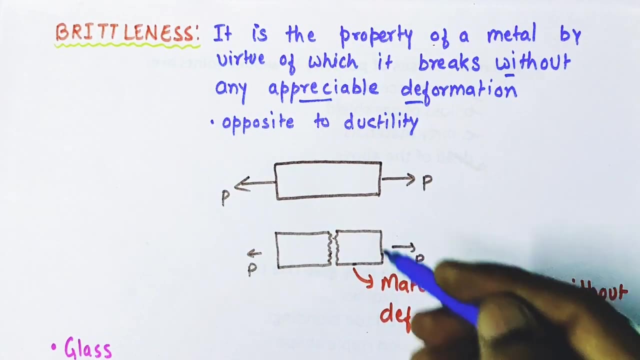 appreciable deformation means if you pull that material, the material will break with very little or no deformation. initially, inductility: the material could be, you know, drawn into thin wire. but here it will not be drawn into thin wire and the shape will also not deform appreciably. 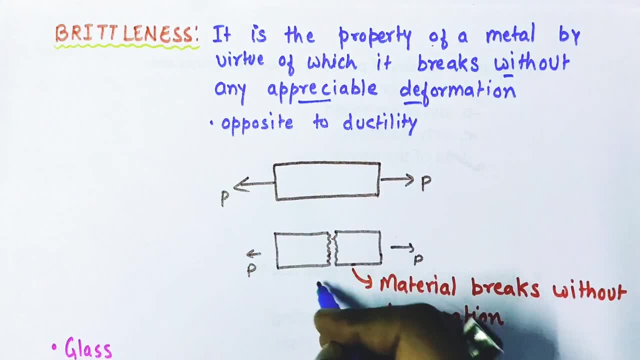 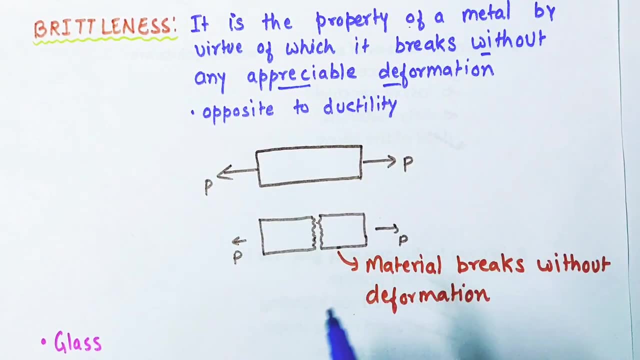 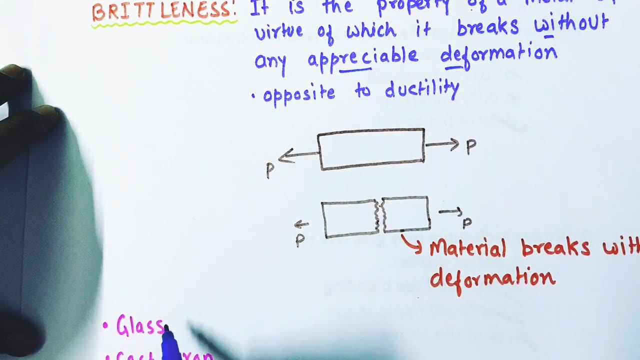 but just you'll, you know, pull that material and that material will break. so in this manner you can call that this material is brittle. material means there is no deformation. without deformation, the material has been broken. so material breaks without deformation is known as brittleness. glass is one of the very 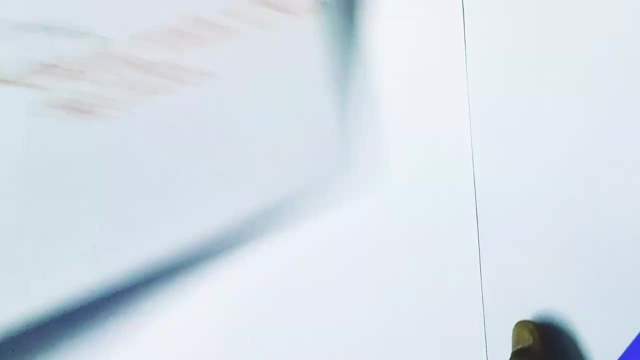 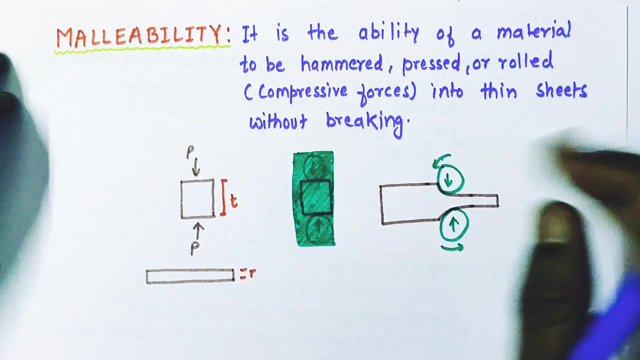 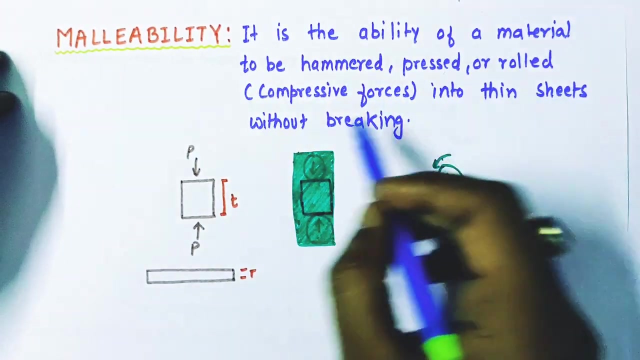 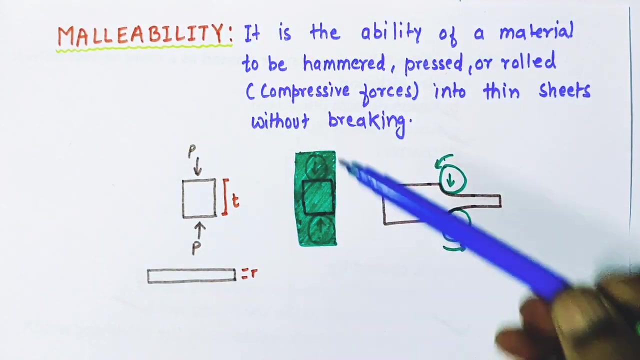 brittle material, then cast iron is also brittle. so after brittleness we'll read about malleability. so malleability, it is the ability of a material to be hammered, pressed or rolled under compressive forces into thin sheets. because without breaking inductility, we are putting, you know, tensile forces, but here compressive forces will come into action. 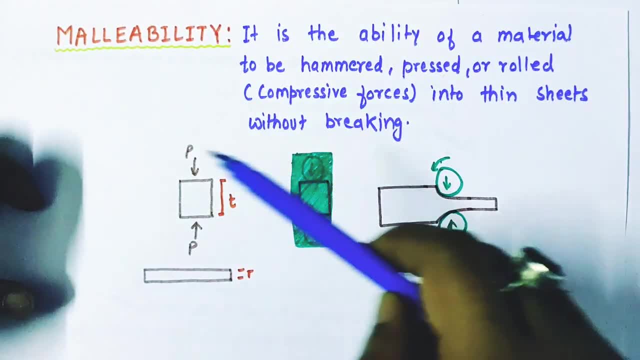 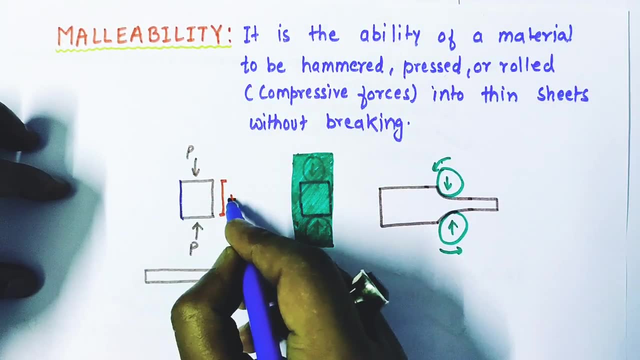 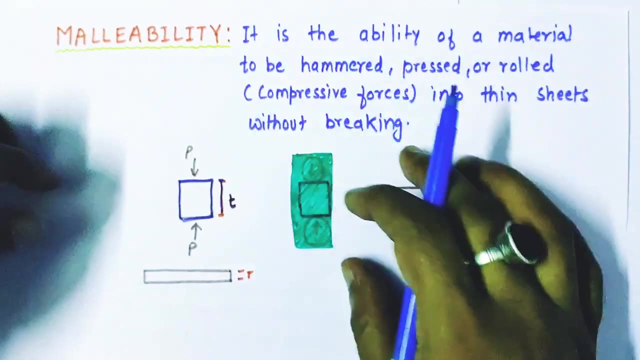 like you'll hammer a material. so upon hammering, that material will convert into thin sheets like here you can see. here you have a material with thickness t. you can see that inside we have this thickness, your material. now, if you apply compressive load from one side or from both sides, so that material 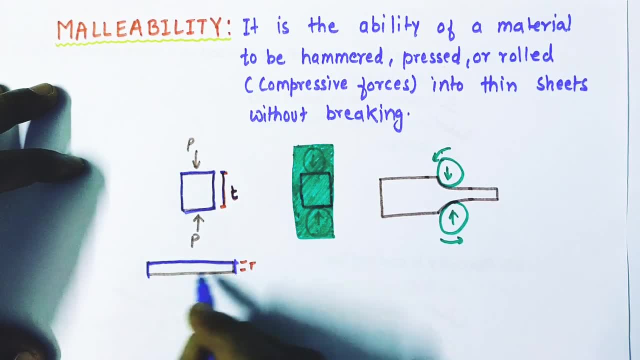 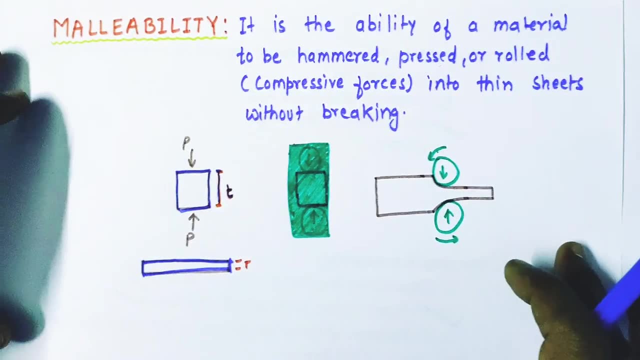 thickness will reduce considerably and it will become a very thin sheet. so this is will be called as that. this material is very malleable means it can be drawn into very thin sheets. here also we have put rollers, and this roller press this material. now, initially, the thickness of this: 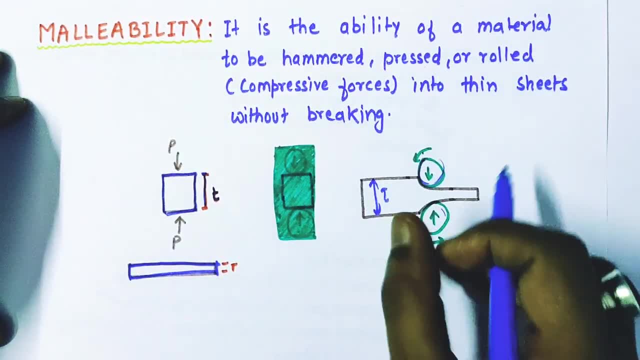 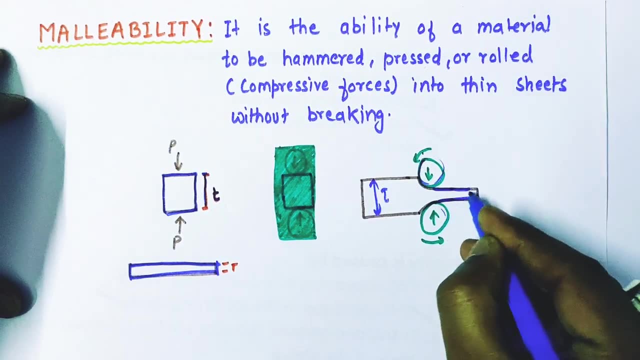 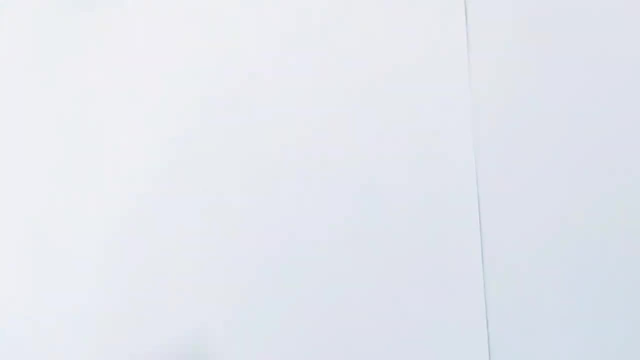 material is this much, but by the application of the compressive forces which has been brought by these rollers, the thickness of this material has reduced into a thin sheet means we can say that this material is malleable. so after malleability we will read stiffness and toughness. so stiffness. 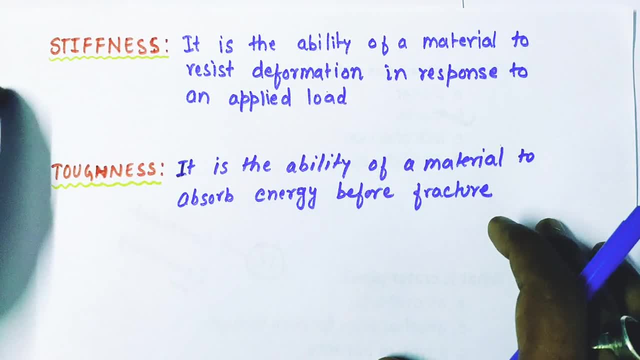 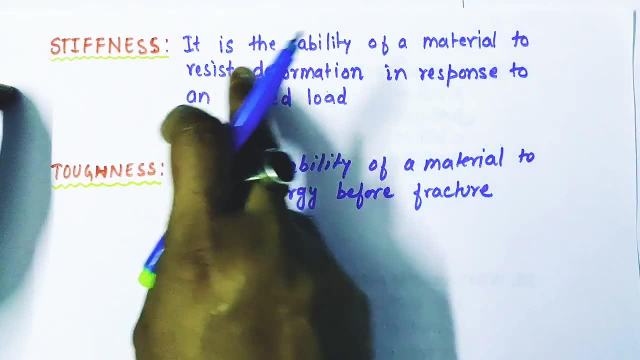 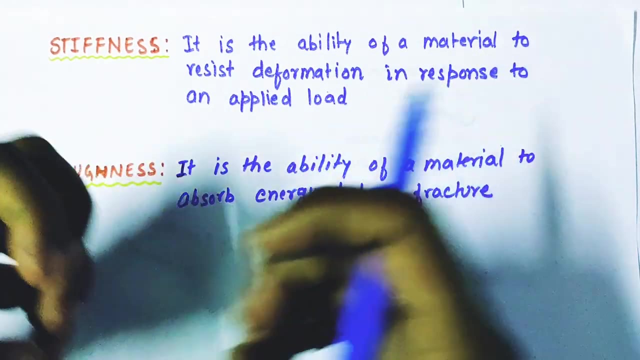 and toughness. many people use it interchangeably, but as far as physics or engineering is concerned, these two are different. stiffness it is the ability of a material to resist deformation, to resist deformation in response to external applied load. so if you apply some external load, the material will try to resist the deformation, and that is called a stiffness, whereas toughness? 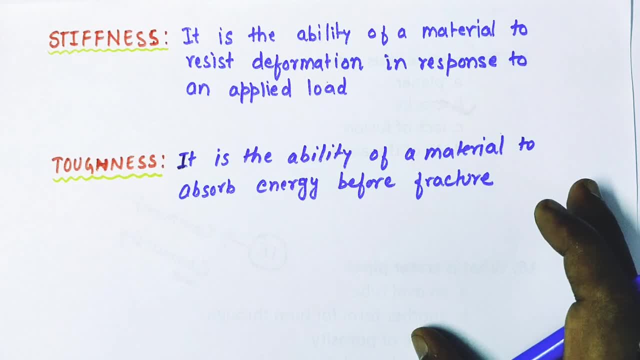 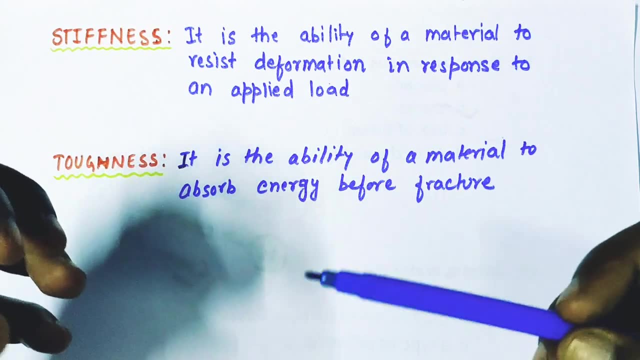 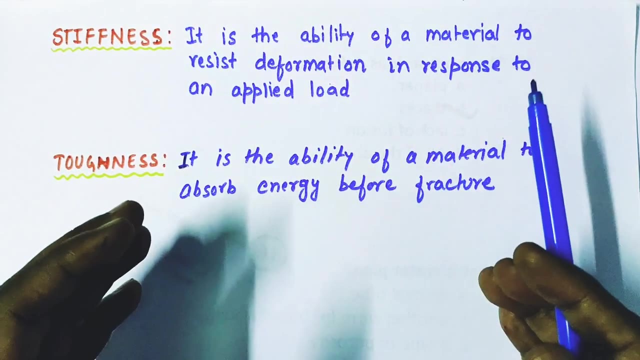 it is the ability of a material to absorb energy before fracture. so when we you will pull the material, it will deform, it will keep on deforming, keep on deforming and finally it will fill. so, before fall, fracture or before fail, the energy which will be absorbed by that material is called as toughness. 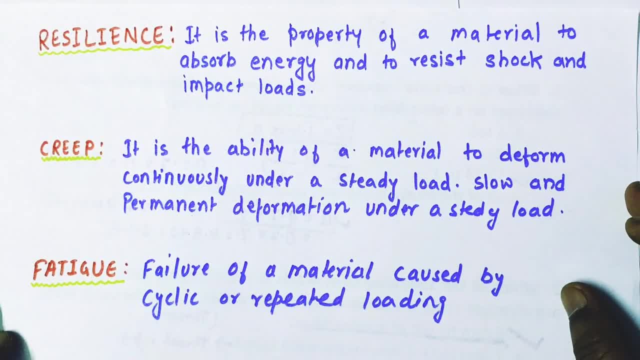 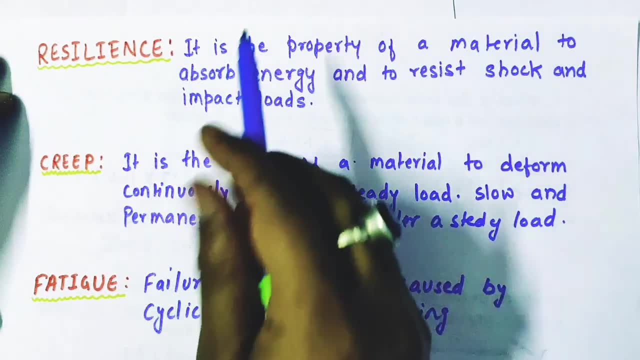 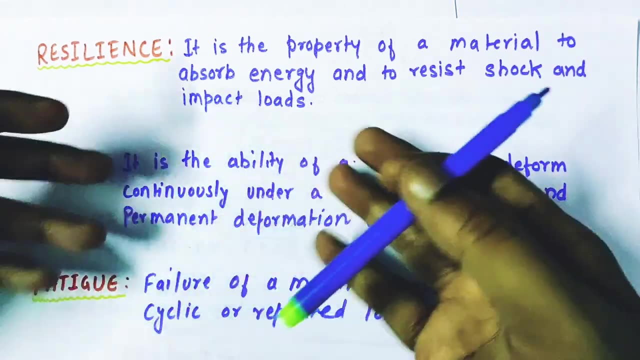 now we'll we understand resilience, creep and fatigue. creep and fatigues are this. these terms are, you know, used in long term. uh, loadings, see resilience. it is the property of a material to absorb energy and to resist shock and impact loads. impact loads are sudden loads, so the more resilient 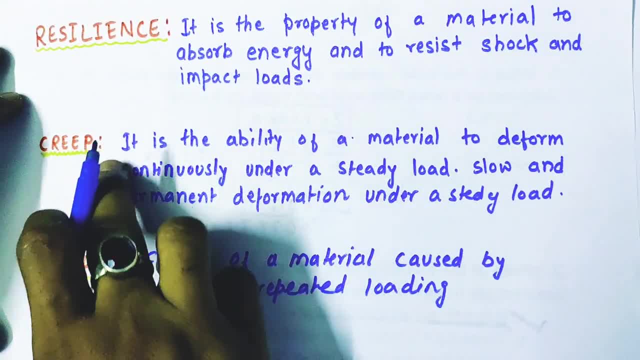 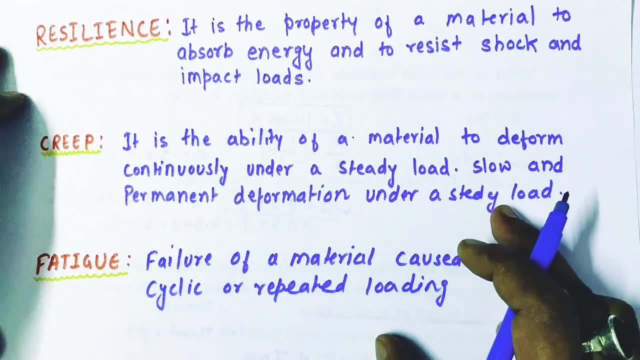 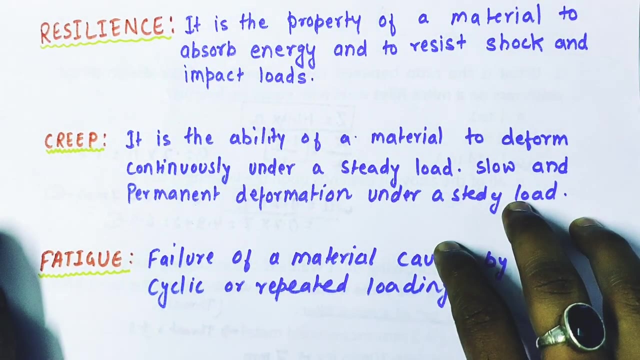 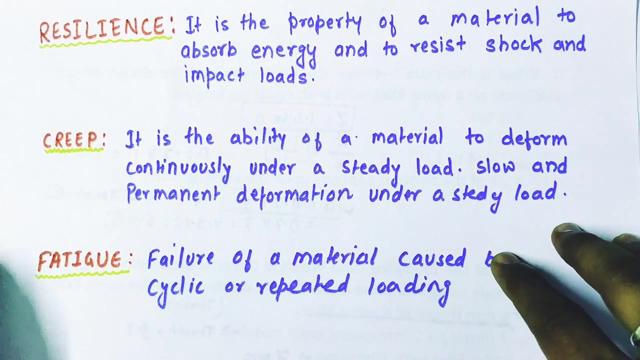 material, it can withstand more impact loads. now creep it is the ability of a material to deform continuously under a steady load. slow and permanent deformation under study load means if you put a steady load continuously on a material, so over the period of time time- long period of time means over the years- the material will keep on, keep on, keep on deforming. so it is. 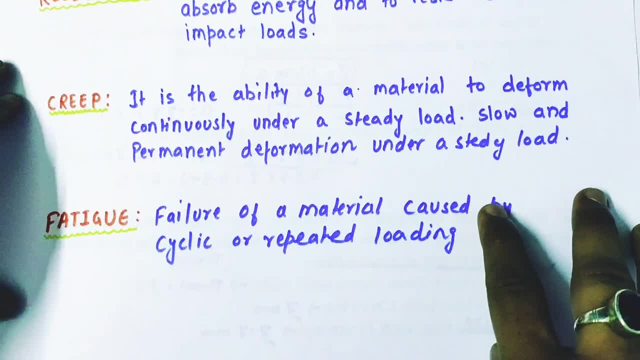 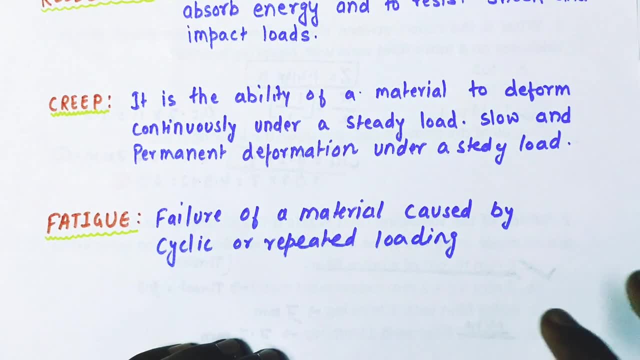 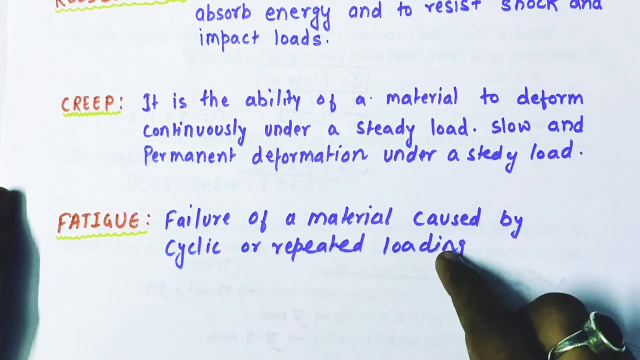 a permanent deformation under a study, load over a period of time, and fatigue. fatigue is a failure of a material caused by cyclic or repeated loading. this loading are very small means much smaller than the tensile strength, ultimate tensile strength. but what happens? due to continuous or cyclic loading, the material fails over a long period of time. so that is called as fatigue. 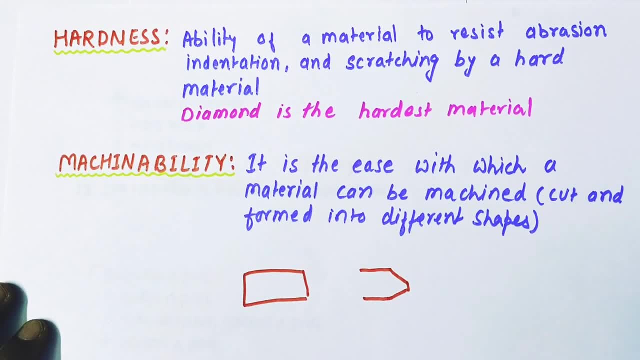 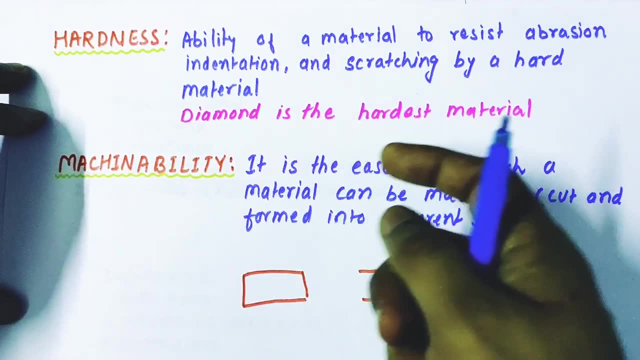 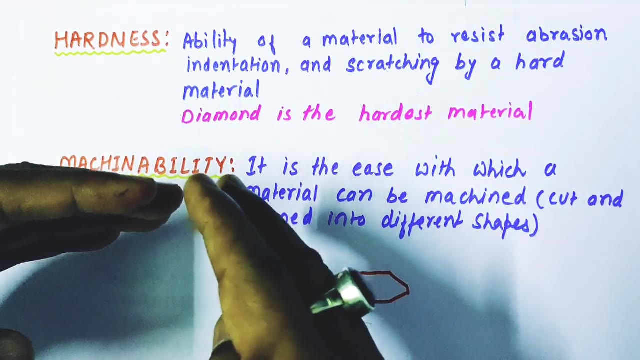 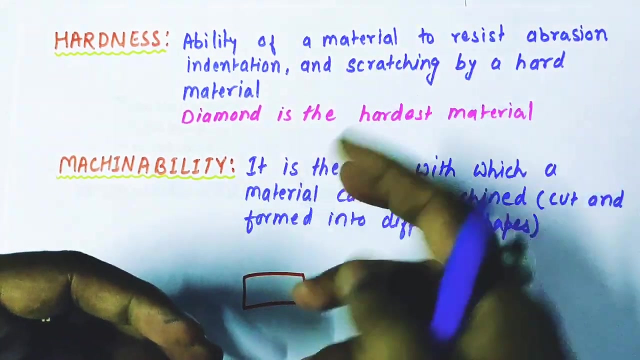 now hardness and machinability. so, friends, hardness, a material to resist abrasion, indentation and scratching by a hard material. if a hard material will try to scratch the material, then the material will show some resistance. so the more resistance the material will be showing to the indentation or to the scratching, the more harder that material. 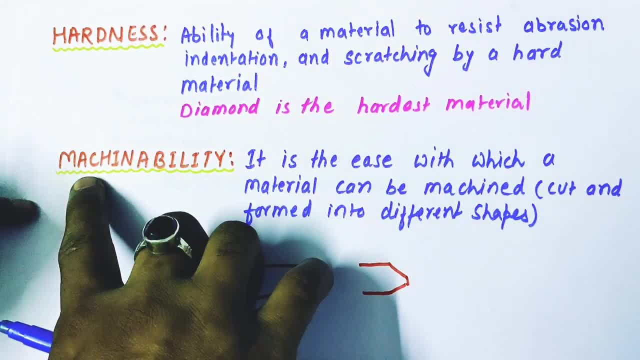 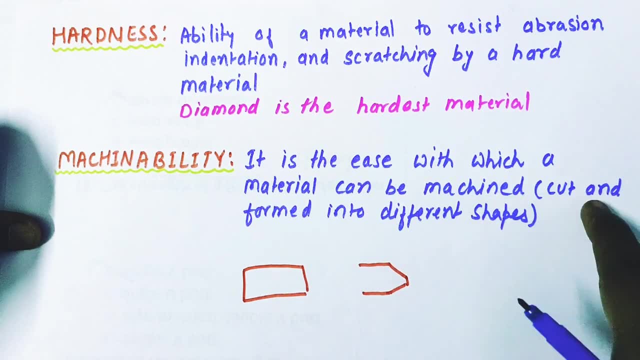 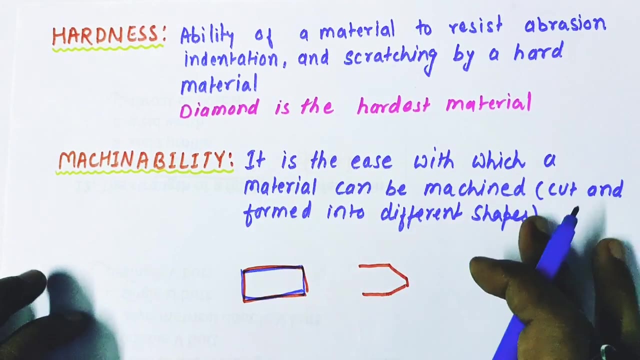 will be like diamond is the hardest material. now, finally, we have come to the last topic, that is, machinability. and machinability, it is the ease with which a material can be machined, that is cut and formed into different shapes, like here: we have a you know component. now we have to make it to. 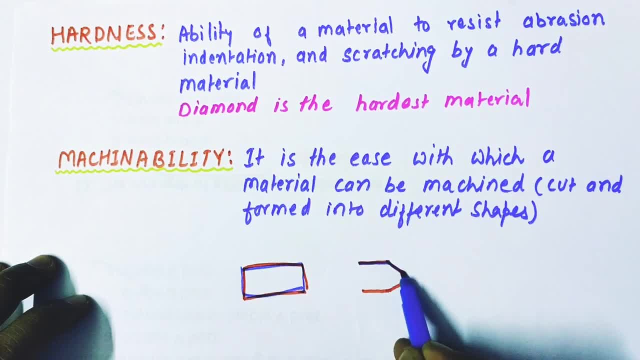 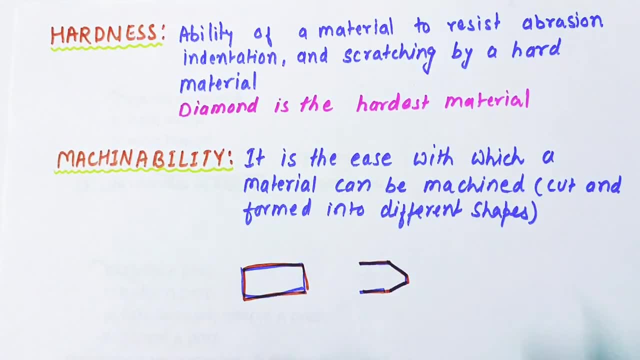 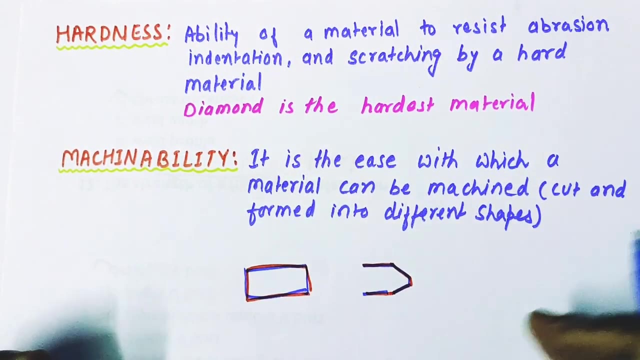 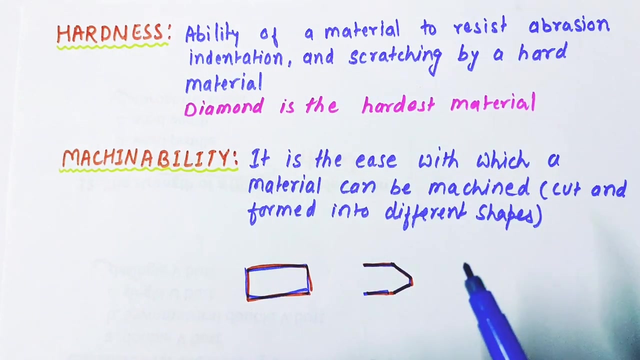 some useful shape so we can convert it to a useful shape with the help of lathe or by some other machine. so the ease with that the machine can be machined and cut and different shapes can be obtained is called machinability. the more a component can be machined, more easily we can call that that component is more machinable.